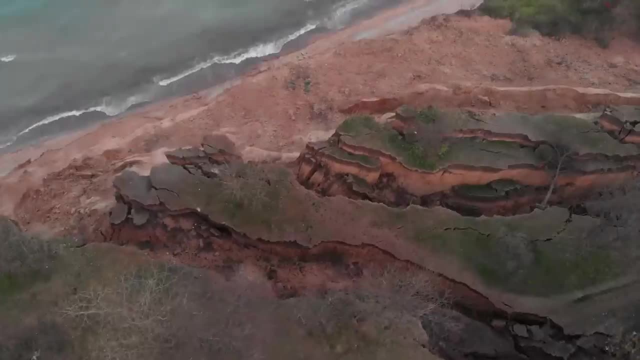 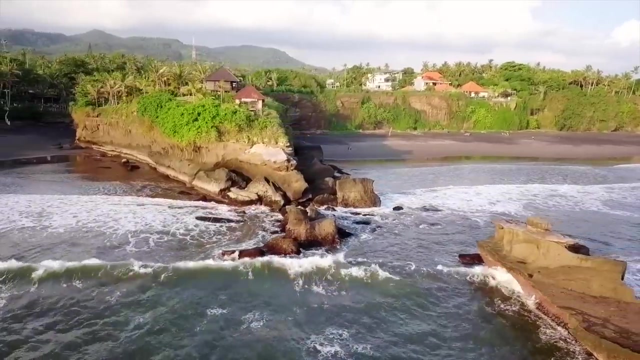 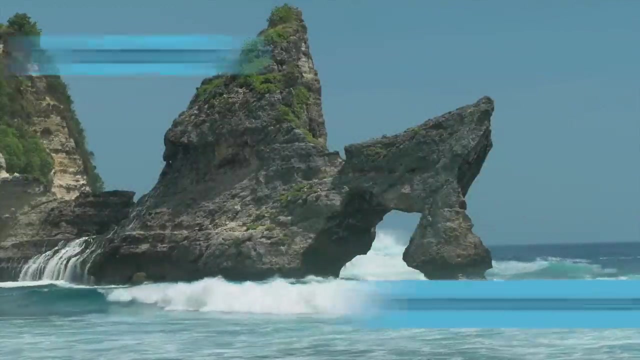 water. This constant process of weathering and erosion along the coastline can create or destroy all kinds of new landforms like bays, caves, sea cliffs and coastal dunes Weathering: There are three main types of weathering. The first is chemical weathering. 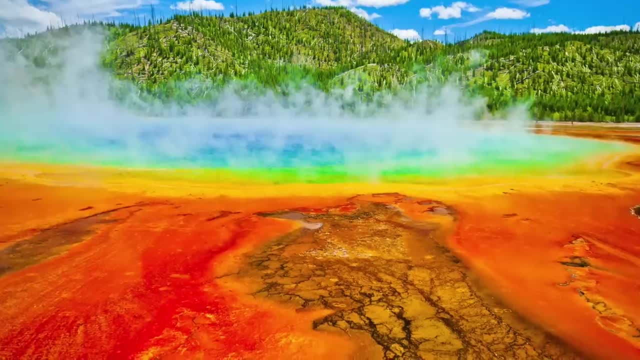 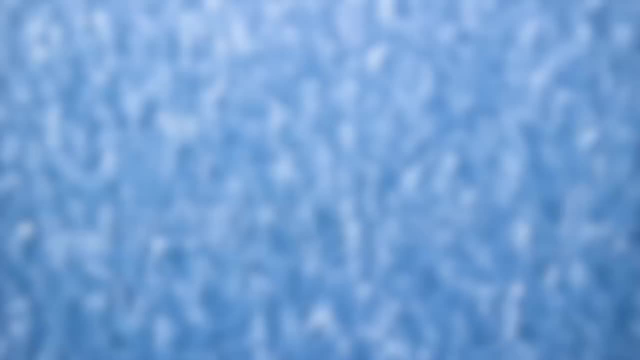 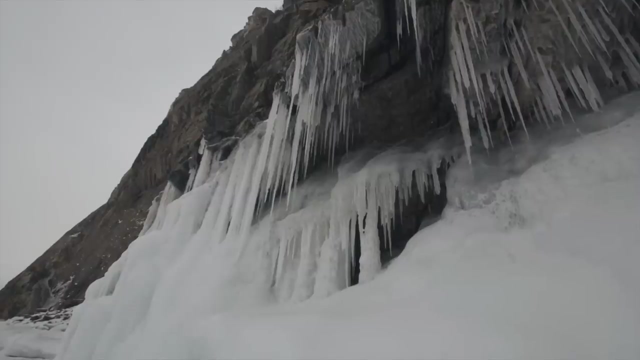 Chemical weathering causes changes to the minerals inside or on the surface of a rock. This process Happens through chemical reactions. Second is mechanical weathering. Mechanical weathering is caused by frost, ice, moving water or heat from the sun. An example is when water seeps inside a 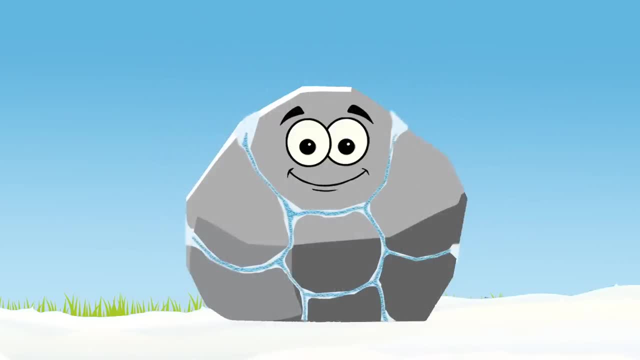 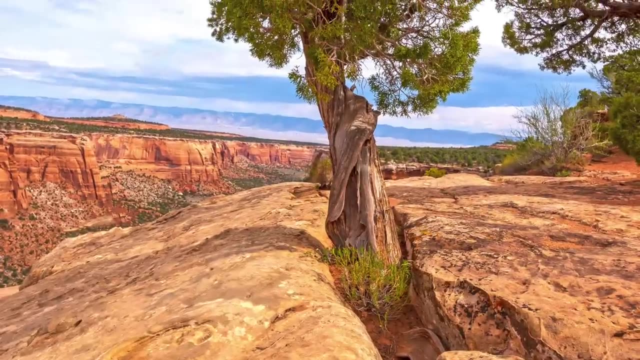 rock and freezes, The frozen water expands, causing the cracks in the rock, which eventually breaks the rock into smaller pieces. The last type of weathering is called biological weathering. Biological weathering, Biological weathering, is the process that occurs when plants, animals and Heh 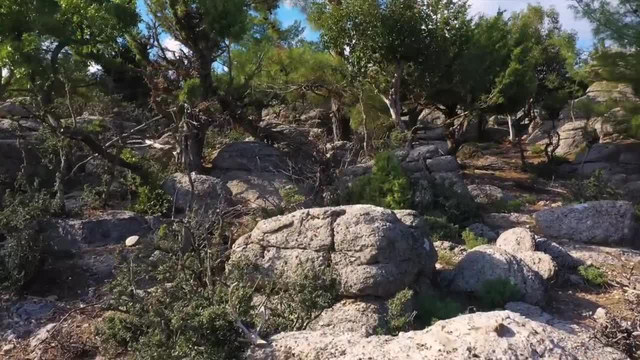 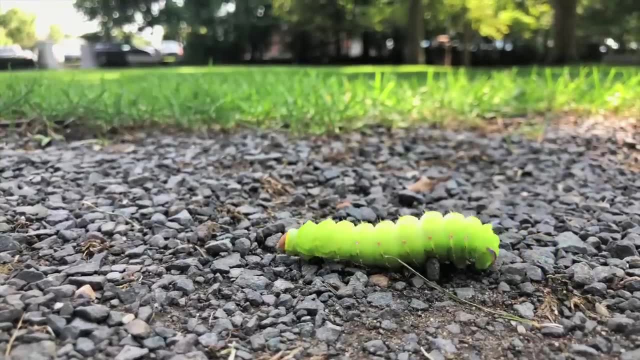 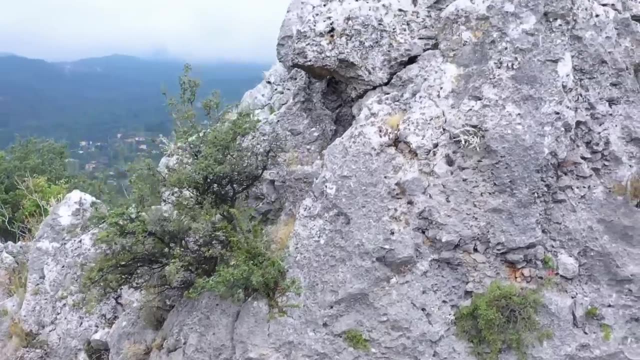 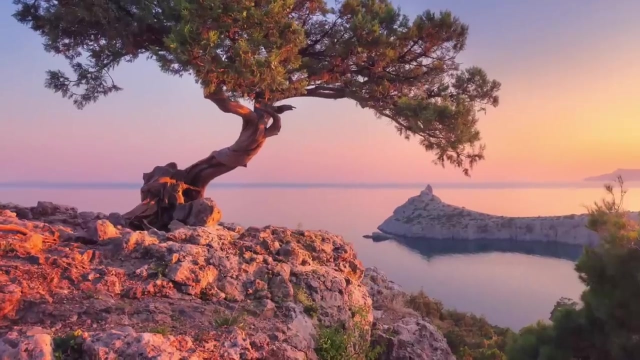 biological weathering and other living organisms caused larger rocks to be broken into smaller pieces. Bat substitute in this example, Worm trees, öldes, mod rewarded Because in both cases the weathering happens because of a living organism. These three types of weathering cause rocks to break up into smaller pieces, which sets this 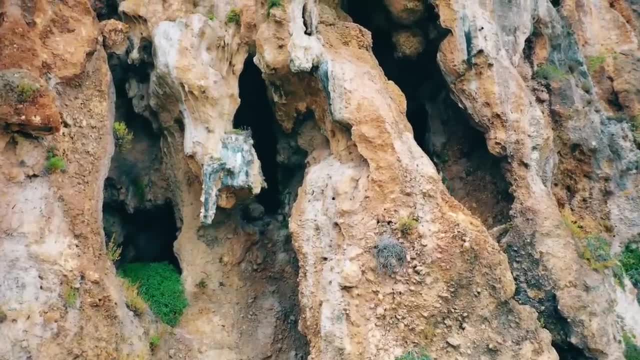 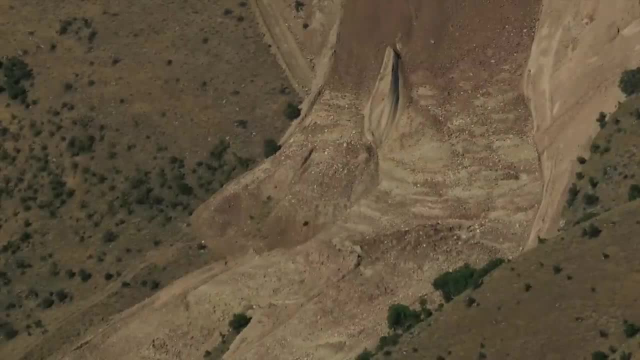 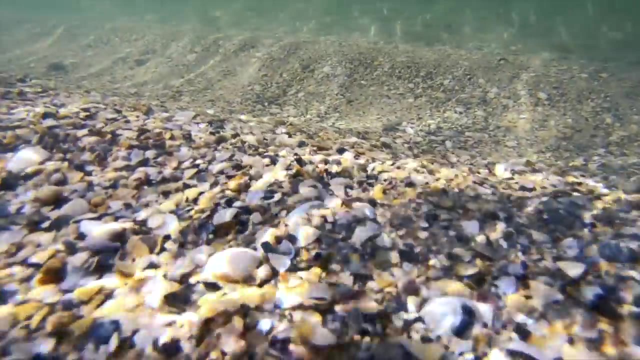 sets the stage for erosion to take place. Erosion: Once weathering has taken place, the smaller pieces of rock left over can begin to move by natural forces. This is the process of erosion. Erosion can happen rapidly or over the course of millions of years. 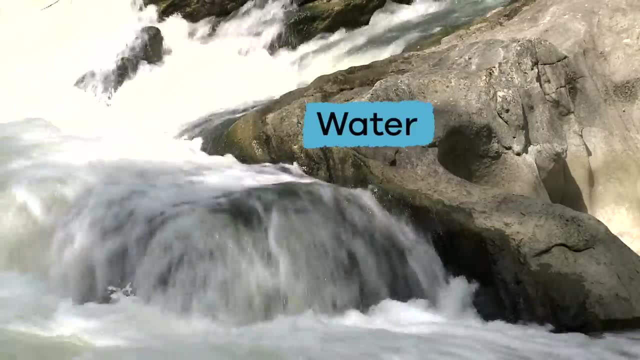 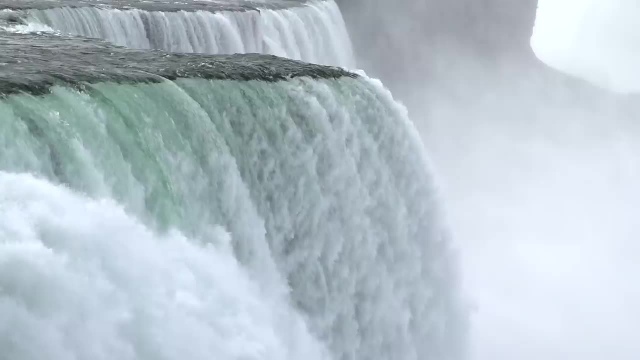 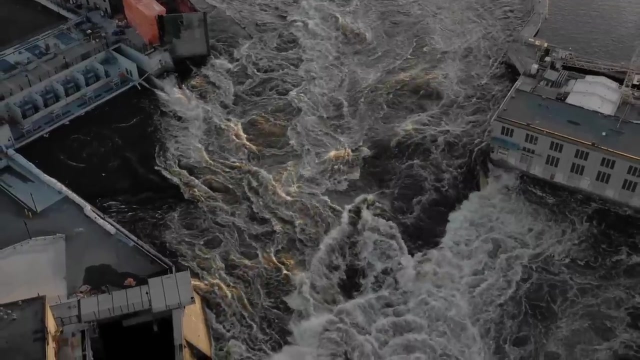 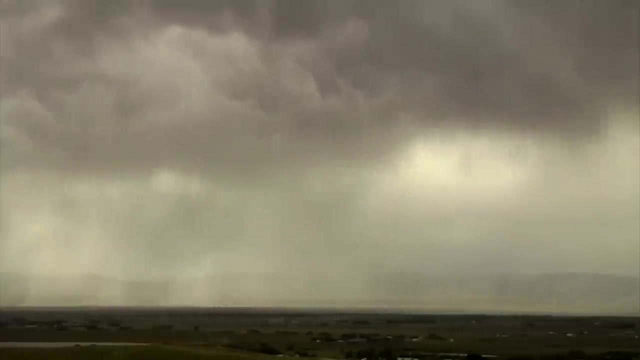 The three main causes of erosion are water, wind and ice, But all different kinds of things can cause erosion to happen. Water can cause erosion through rain, rivers, waves and floods. These natural events and landforms cause erosion as the water crashes into the earth. 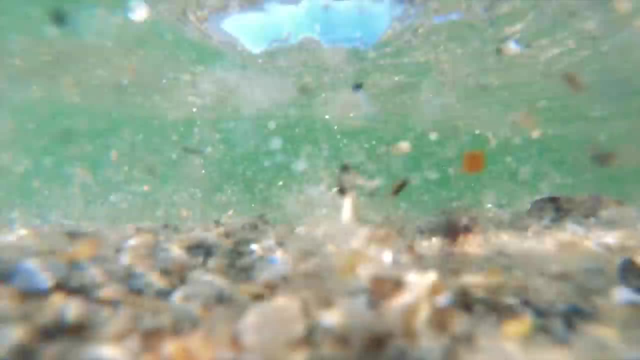 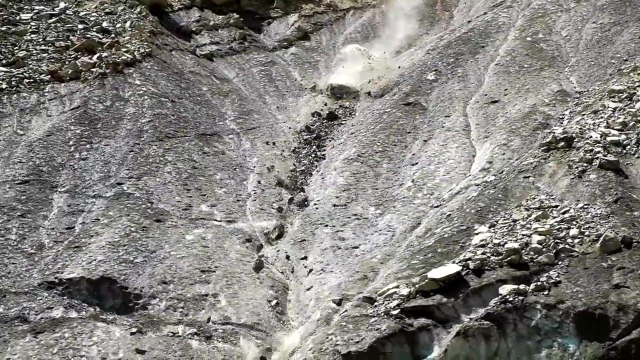 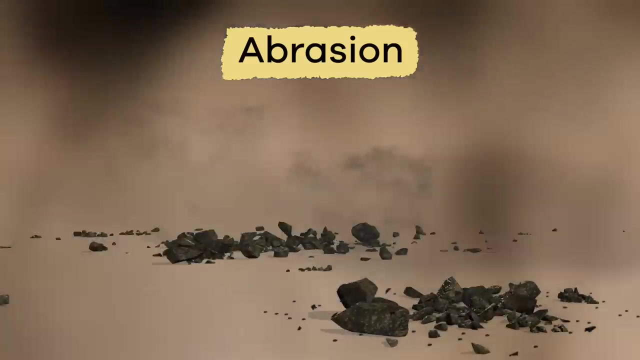 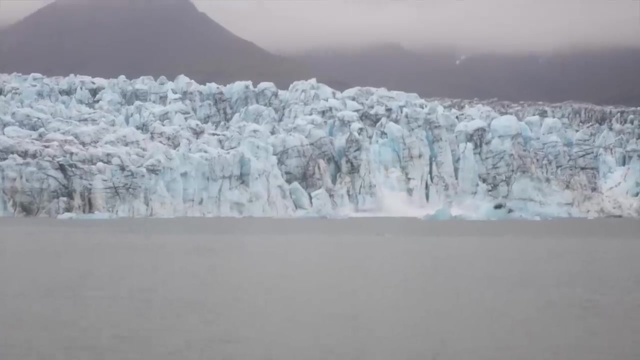 gathering and moving particles along the way. Wind picks up and carries loose particles and dust, Sometimes crashing into other landforms and breaking off more particles. This process is called abrasion. There are massive formations of ice called glaciers. These icy masses move and shift to cause erosion. 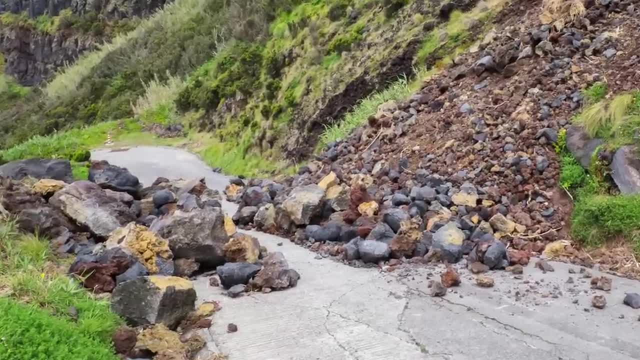 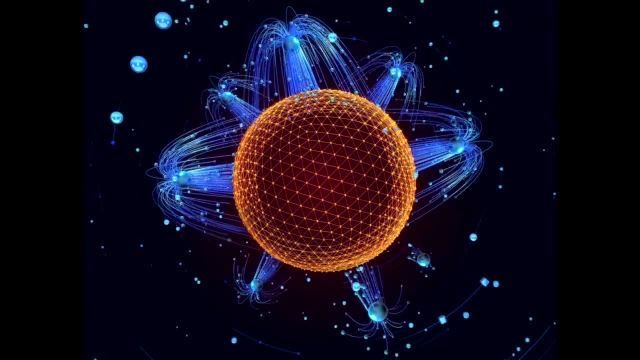 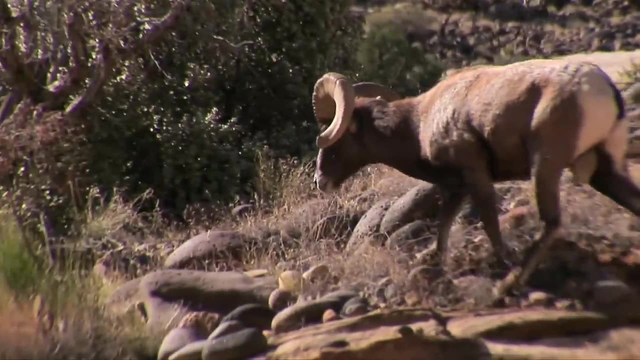 The forces of gravity can cause erosion too. Think of a landslide or a rockslide falling down the slope of a mountain. This happens because of earth's gravity Or a gravitational pull. Living organisms like plants and animals cause erosion as they move particles from place to place. 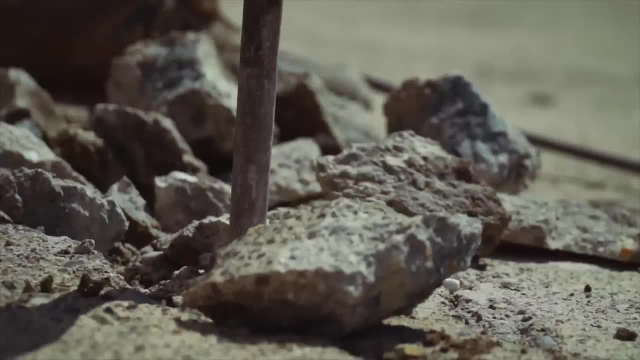 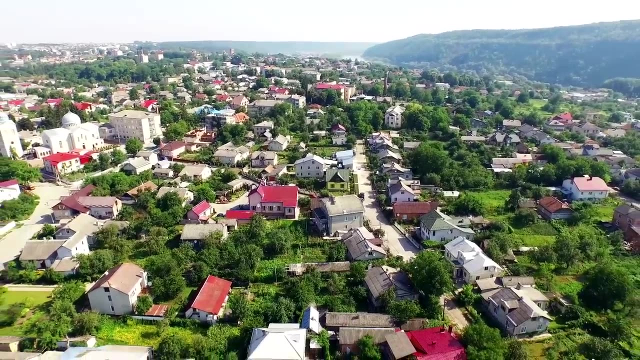 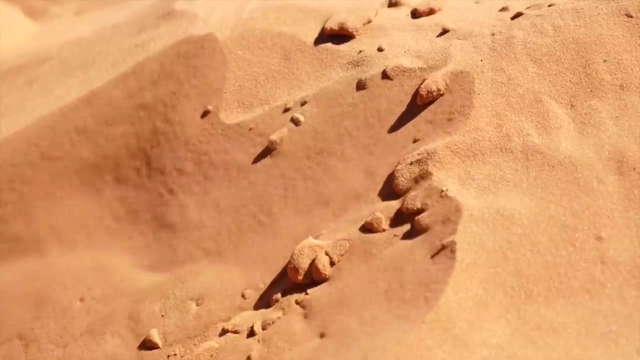 Even humans can cause erosion. Although not naturally occurring, humans can cause erosion through farming, cutting down trees and building roads and buildings. Everything you do to the earth can cause all kinds of changes Through erosion. the sand pebbles. 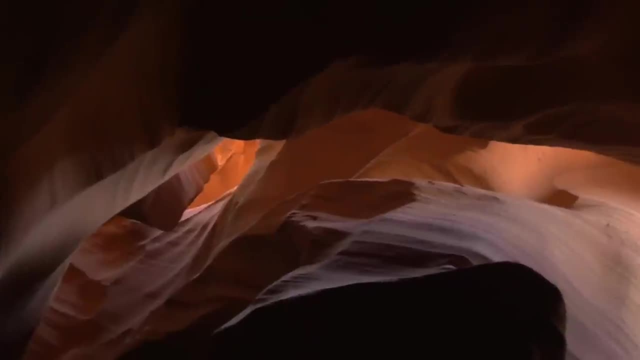 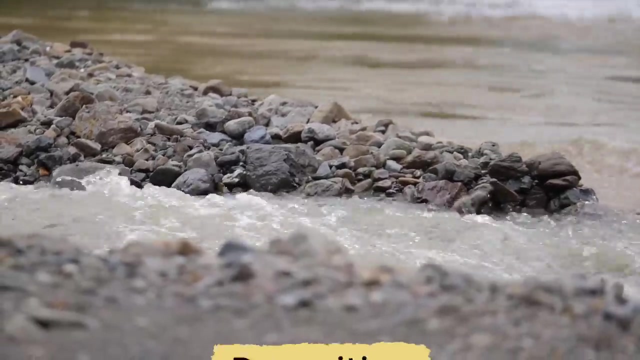 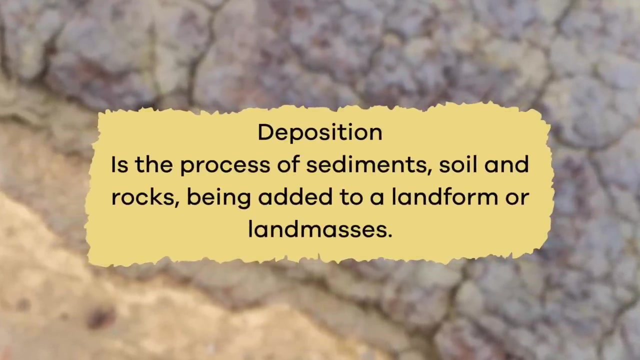 mud or other pieces of sediment might eventually reach their final or temporary resting place. When the sediment rests or deposits, it is called deposition. Deposition is the process of sediments, soil and rocks being added to a landform or land masses. 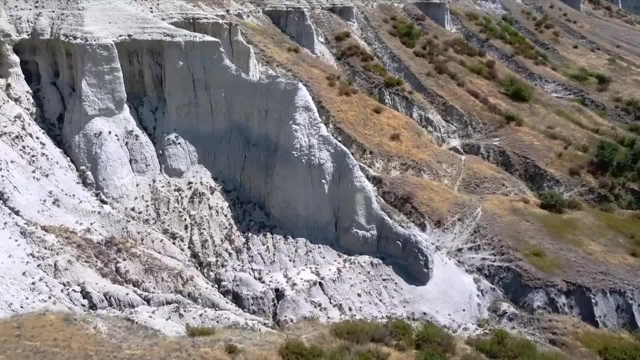 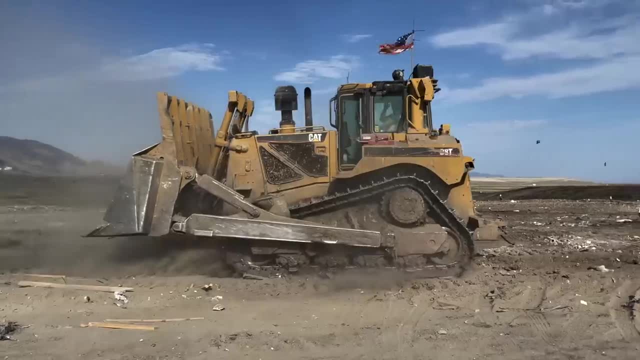 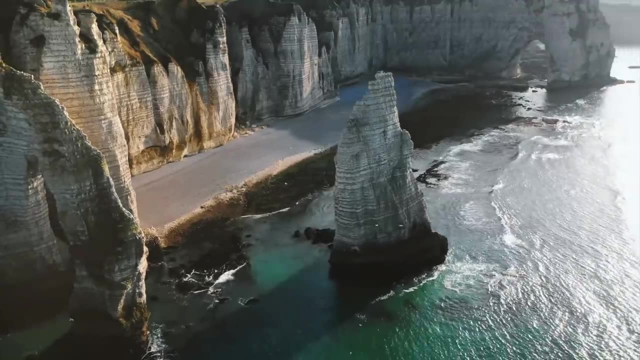 It marks the process of erosion coming to an end and possibly results in the forming of a new landform. But remember, weathering and erosion are happening all the time, So when one of these processes has finished, another process just might be starting. 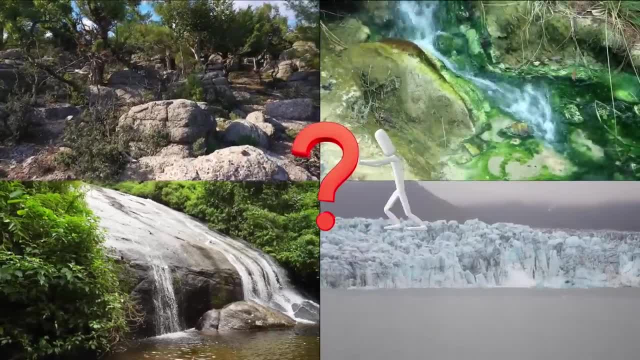 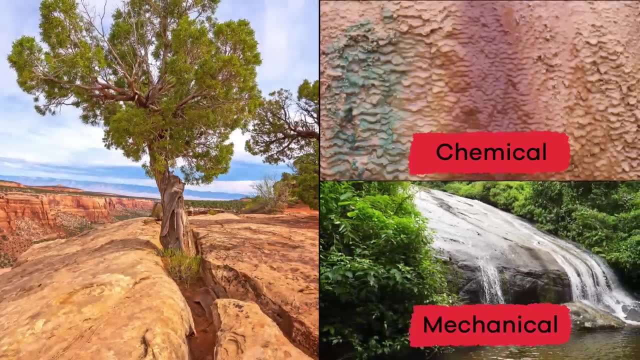 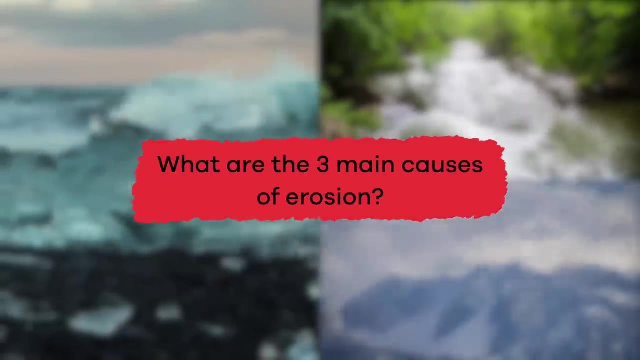 We've learned a lot of new facts, so let's review. What are the three different types of weathering? Chemical, mechanical and biological? What are the three main causes of erosion? Water, wind and ice? What kind of weathering happens? 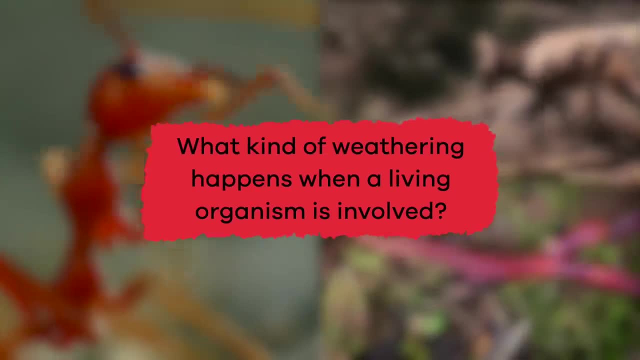 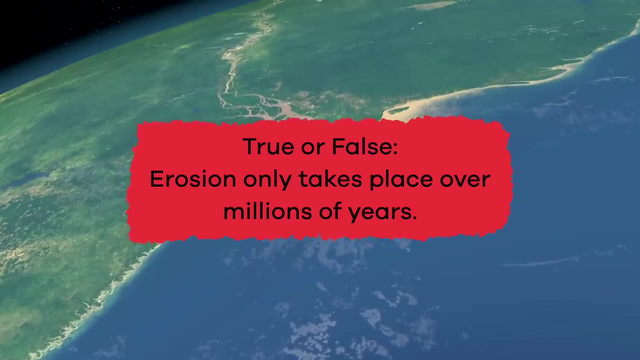 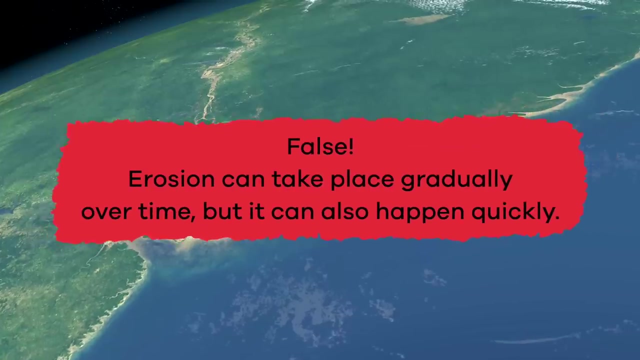 when a living organism is involved, Biological weathering, True or false Erosion only takes place over millions of years. False Erosion can take place gradually over time, but it can also happen quickly. What are the three main causes of erosion?